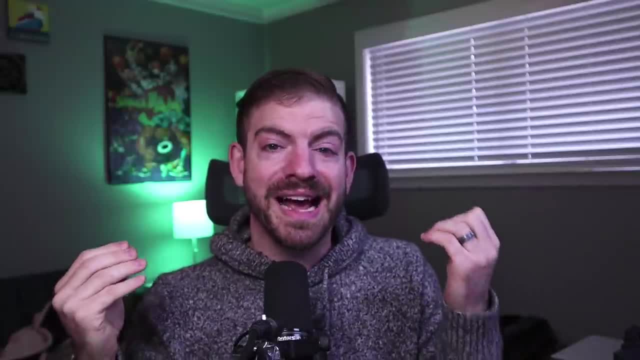 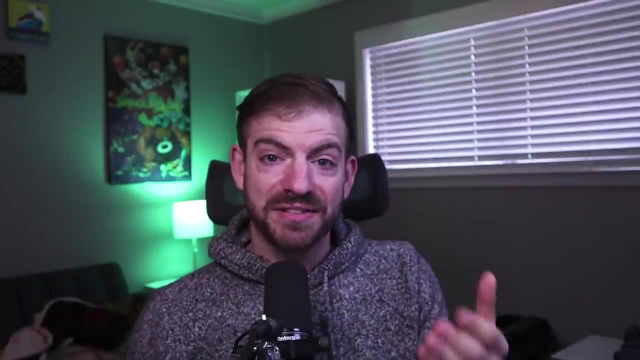 the number 32 inside of it and I check to see if I have a string with the number 32 inside of it. but objects are not looking at the values inside of the objects, it's looking at that object in memory. does this actually point to the same object and memory? And if that stuff doesn't? 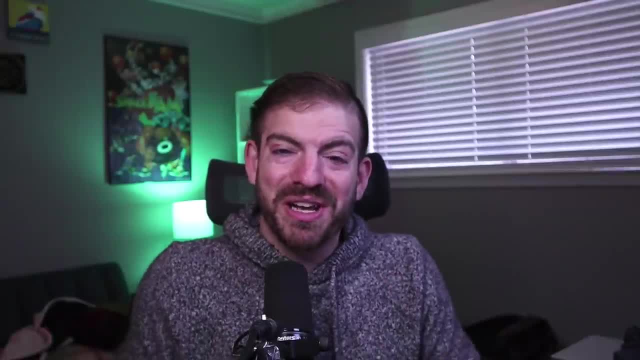 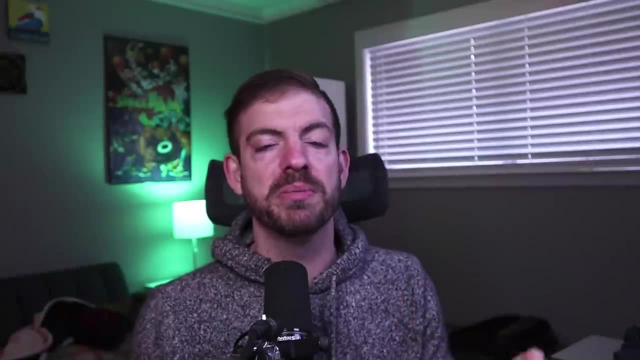 make any sense to you right now. that's why this is number one on my list, because it's very important in JavaScript knowing how the double versus triple equals works, and then knowing how primitives versus objects and basically everything- arrays and classes and all those are objects. 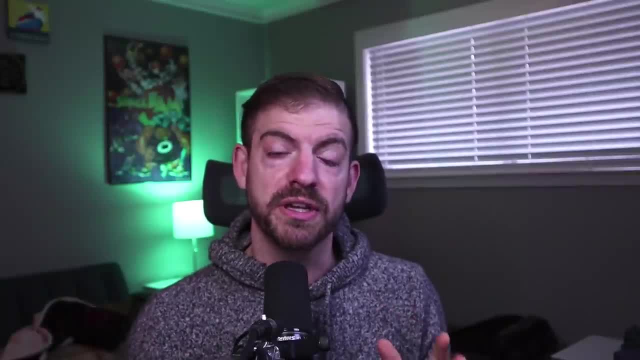 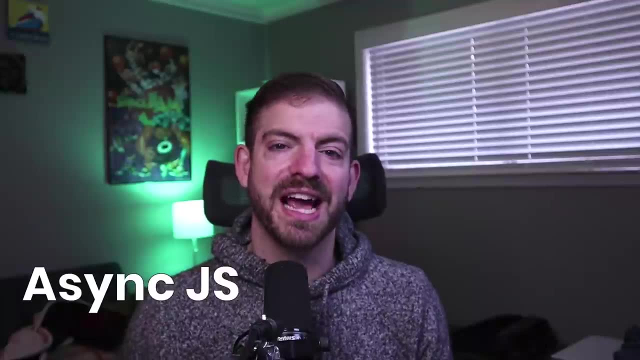 So understanding how those compare in terms of equality is really, really important. Now, number two on my list- and I've done an entire video on this- is asynchronous JS. how does JavaScript run And how do you interact with asynchronous JavaScript? 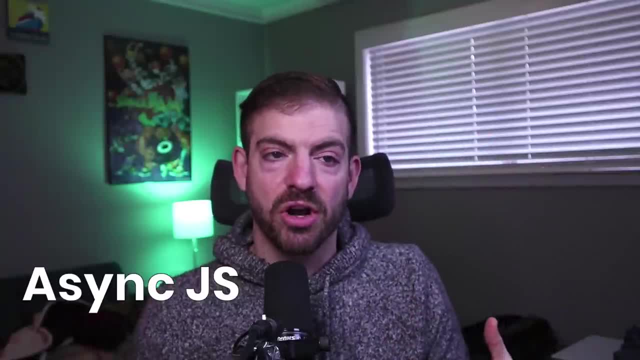 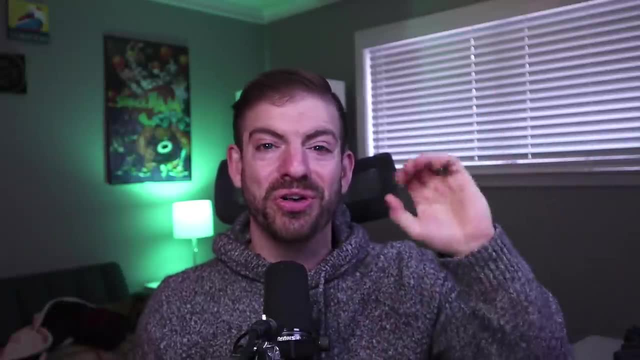 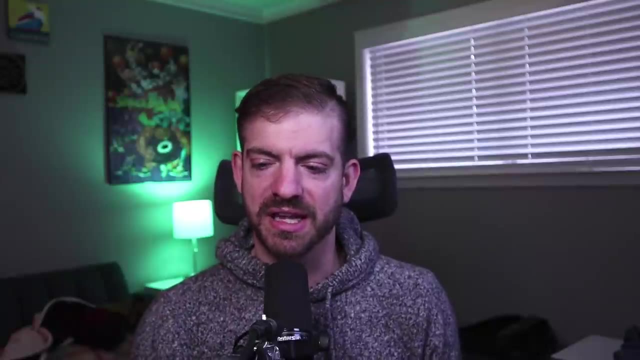 Now this started with callbacks and there's still a lot of callbacks. but you call a function and then as a parameter you pass a callback function. that function is what will get called when that thing finishes doing its work, I guess. So the callback function was kind of the original. 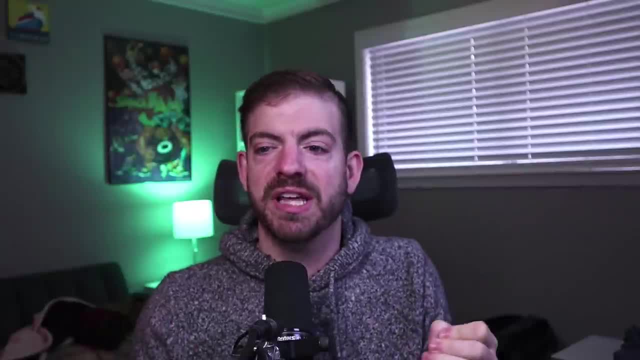 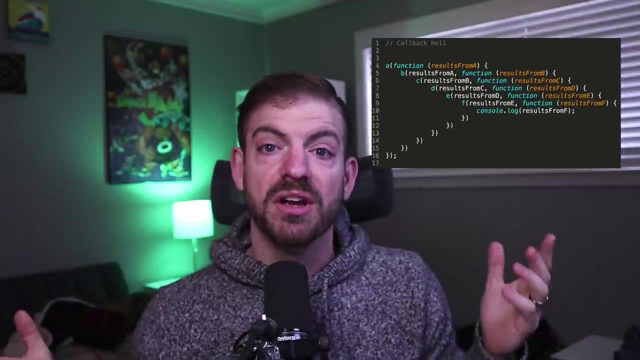 way that we would do asynchronous JavaScript. And then people started to look at it And they said, hey, this can get kind of ugly once you have callbacks inside of callbacks inside of callbacks and you have what's called callback hell. So then they went to promises and that enabled. 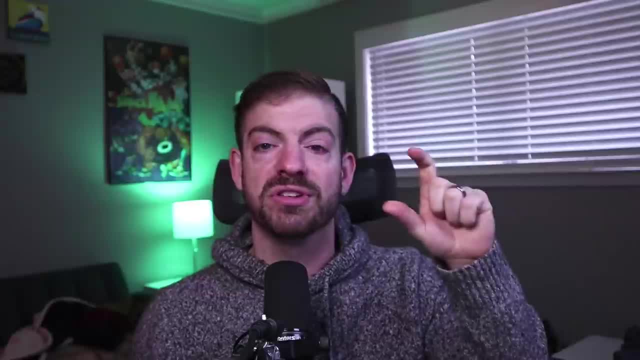 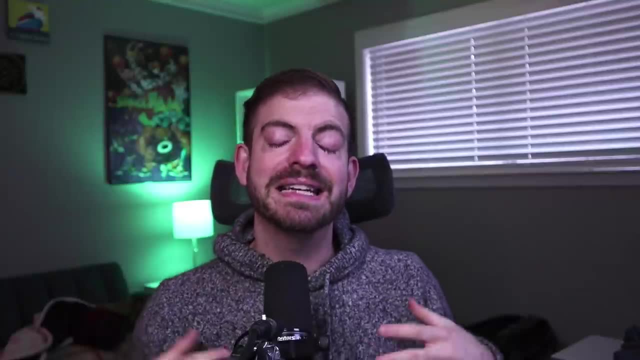 the dot then and dot catch. So a dot then would handle your successful response from a promise, a dot catch would handle the errors coming back from a promise. And then, additionally, they added on async await syntax to match things that are available in languages. 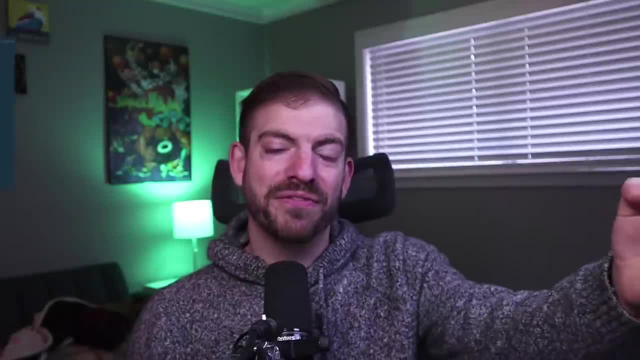 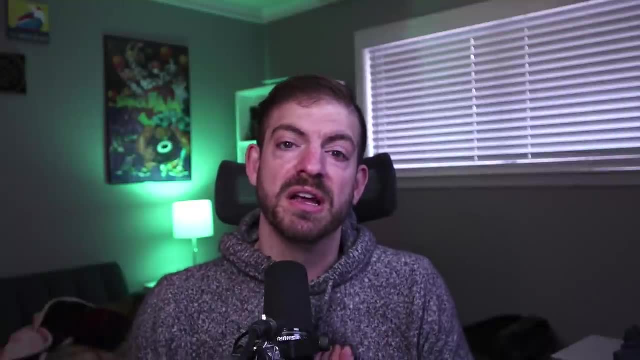 like C sharp. So what this allows you to do is kind of wait for the actual data to come back in line in your code, So you're not having to write a dot, then dot catch, which is my favorite syntax. Again, if you want to learn more about the different ways that you can run asynchronous, 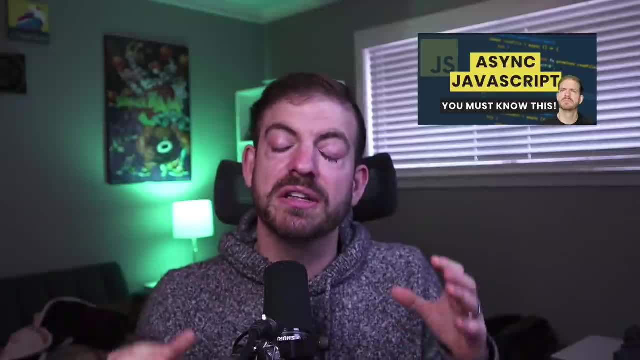 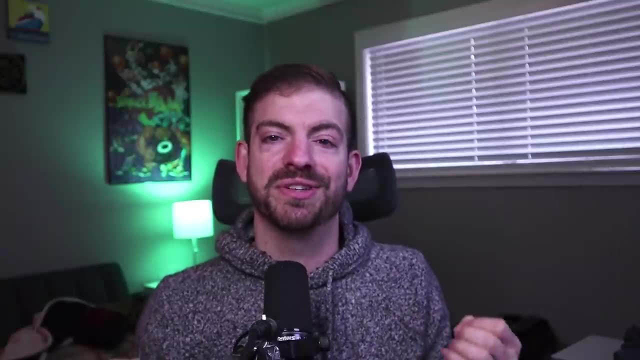 JavaScript, check out that video, But just know that everything are a lot of things that you'll do in JavaScript come from or are asynchronous, So you need to understand how asynchronous stuff works: when to handle a promise, when to do a single weight, all that kind of stuff to make. 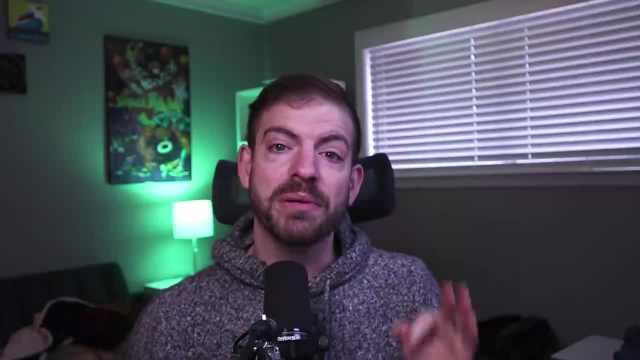 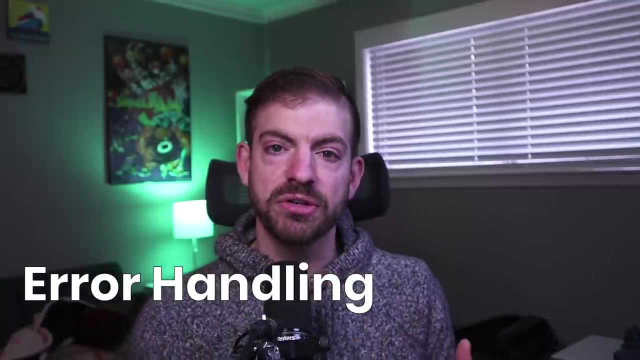 sure that you really understand what is going on, All right. number three is error handling, And this is maybe a little advanced for people that are that are new to JavaScript, But I think this has several different implications And error handling could mean a lot of different things. For example, 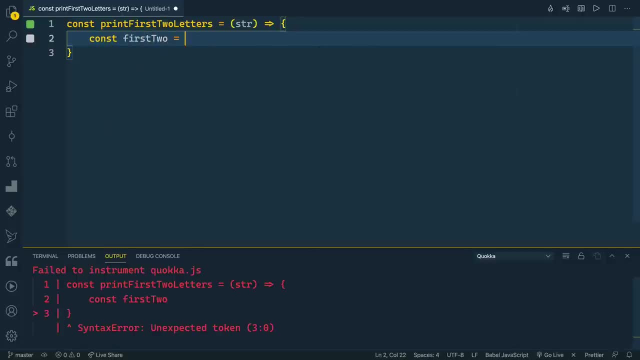 if you define a function that accepts a what you assume is a string, in JavaScript, there's nothing actually guaranteeing that someone's going to pass you a string. they could pass you a number. So then, if you try to access a string, you're going to pass you a number. So then, if you try to access, 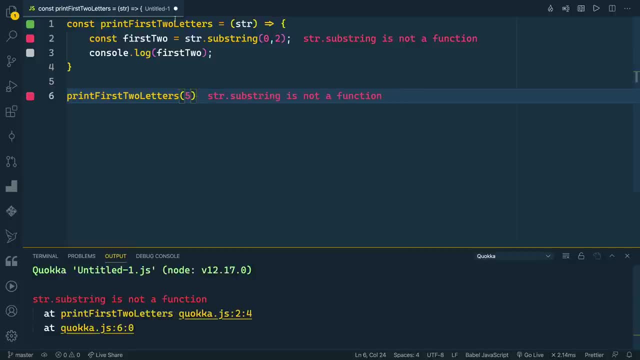 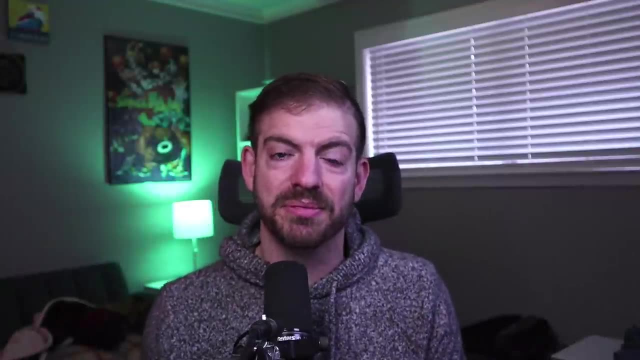 the substring method on that thing, on that parameter, it's not going to work because it's actually a type of number. So you have to prepare yourself for that. you have to think about how can really, how can people mess this up, Because there's really no structure in JavaScript which is the 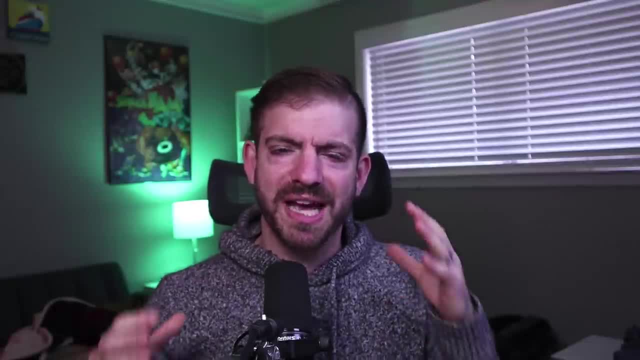 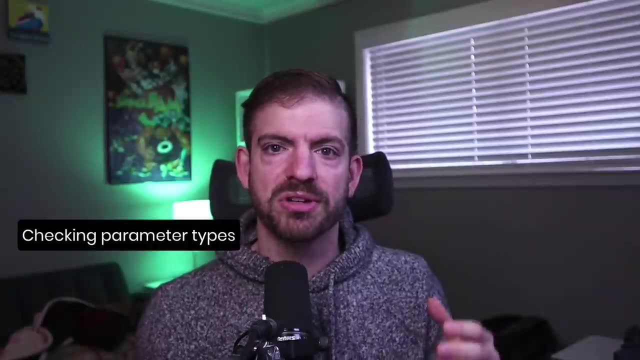 bright side and the downside sometimes. But you have to kind of put yourself in that mindset of how can these things go wrong And, if so, how can I fix it? So, checking the types of your parameters, checking that you actually have data there, that they're not passing null and undefined, or 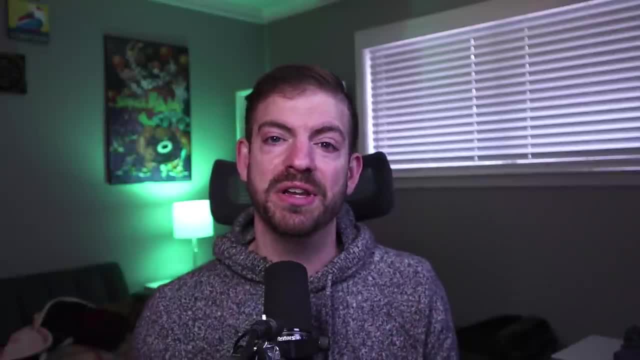 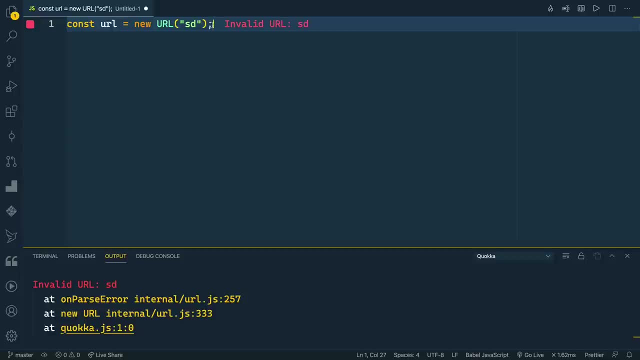 something like that. Another thing is that you can actually do a lot of things in JavaScript, especially if you're running like a node application And one of the more recent feature or versions of node it will shut down your server completely if you don't handle the error. 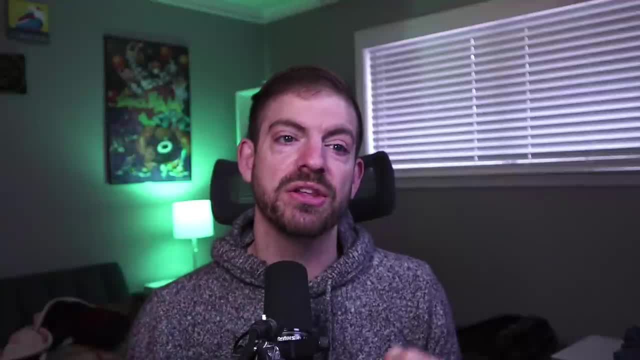 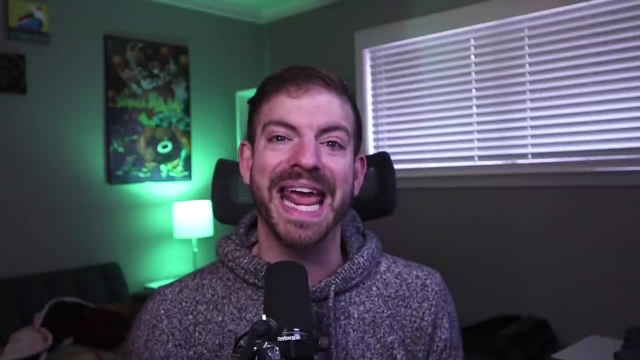 So anything that can throw an error, you need to be able to handle that using a try, catch Again. also think about writing defensive code, preparing yourself for things that can go wrong And handling them nicely yourself so that your application doesn't crash. So error handling. 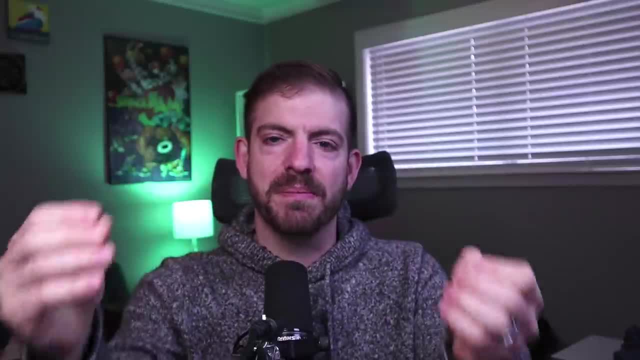 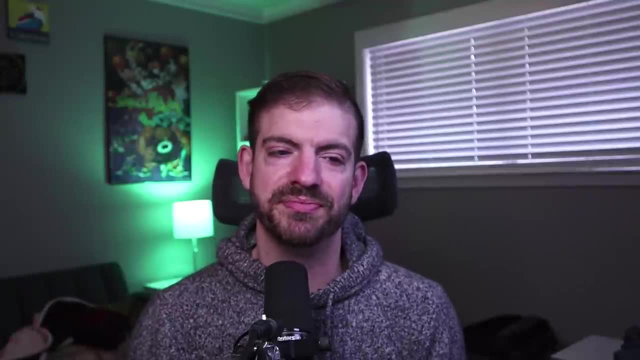 super, super important- has some different implications, And a lot of it is just the mindset about how you think about the code that you write to make sure that you're protecting yourself against things that could go wrong. All right, next up is ES six syntax. So ES six or ES. 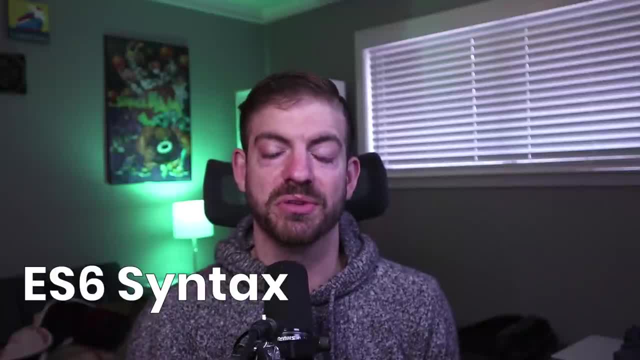 2005 was a really big version of JavaScript. there was lots of things that came in that new version of JavaScript And because of that, that was a really big version of JavaScript And because of that, that was a really big version of JavaScript And because of that, that was a really big version of. 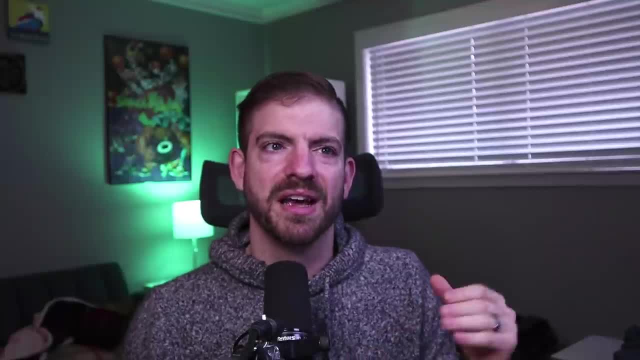 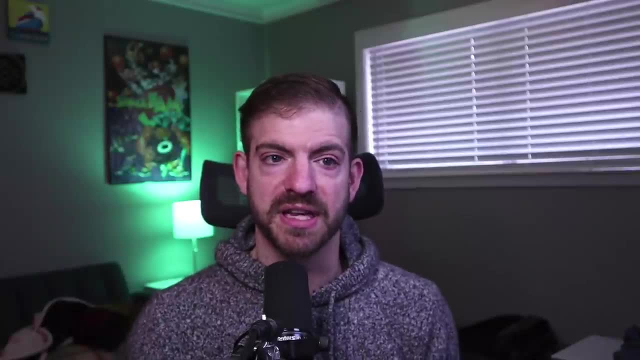 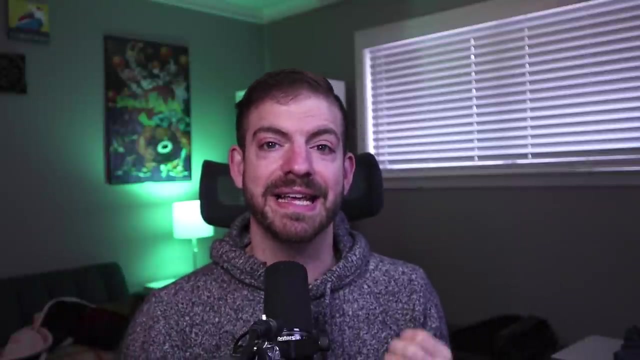 ES six. So that has really kind of been the limiter, for me at least, of kind of like a regular older JavaScript versus newer JavaScript. And if you look at things like react, for example, or a lot of the tutorials that you'll see you're going to see a lot of ES six syntax. 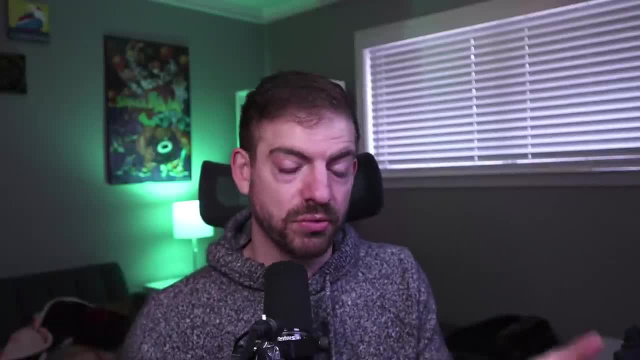 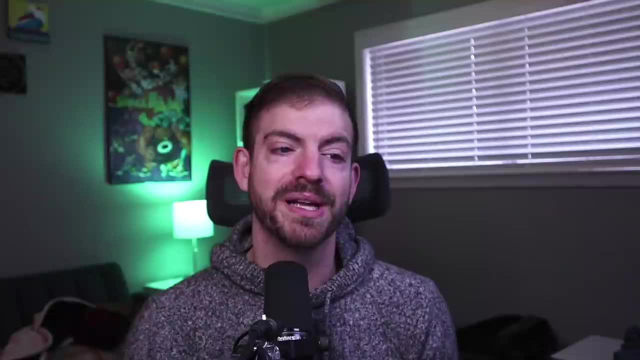 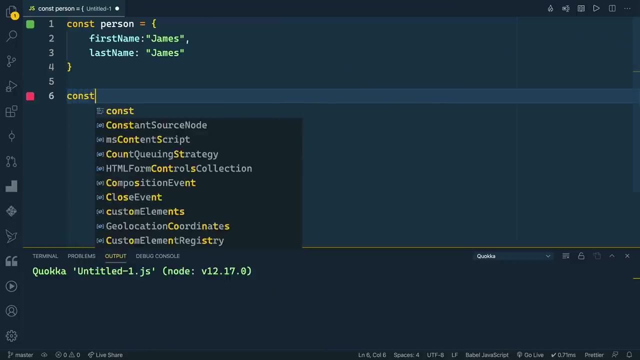 inside of the JavaScript that you see or watch or read on a blog article And if you aren't familiar with that you can kind of become lost. So here's a couple of key features from ES six. syntax that I mean destructuring- is a big, big one. So if you wanted to grab a property off an object, 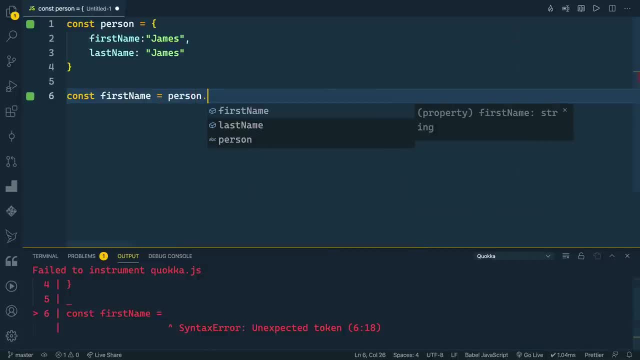 you can do that right in line with a little code snippet And you can destructure multiple properties. you can destructure from arrays. this is used with the use state hook a lot in react, for example. So destructuring is really nice. Also the spread operator. 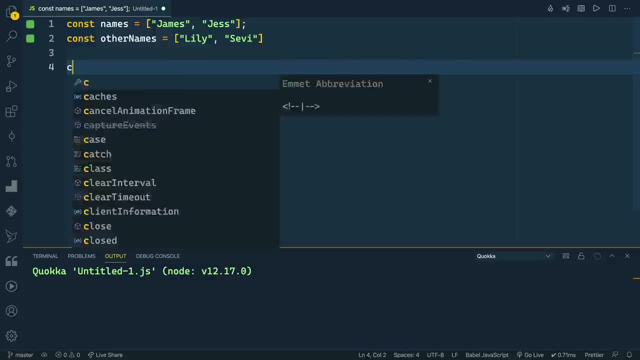 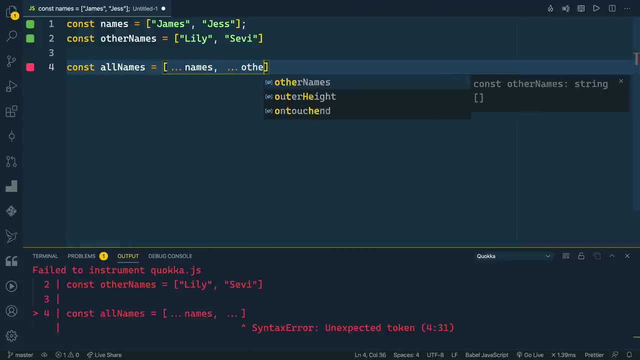 the spread operator allows you to take all of the items in an array, for example, and spread them out, So you kind of get access to them individually. it's useful for passing items in an array as parameters to a function, So you can spread out the items in the array. 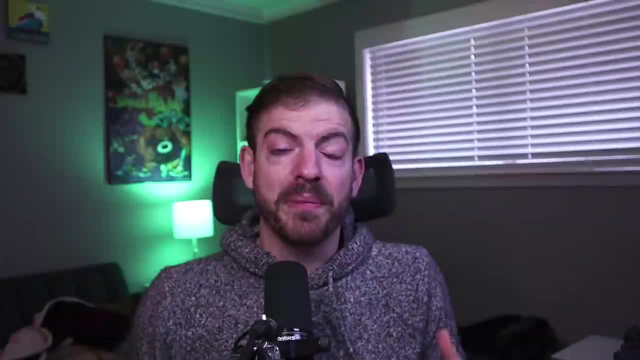 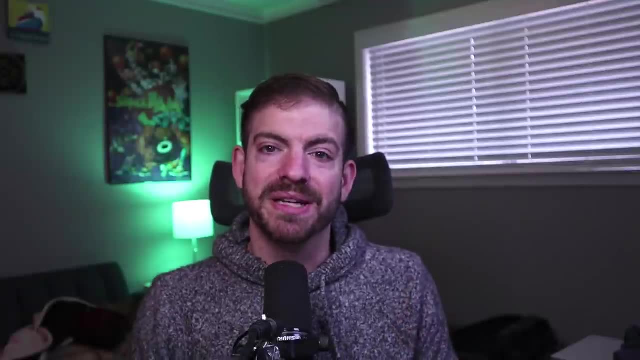 and pass them as individual parameters to a function. It's useful for making copies of arrays, And it's not just for arrays, it's also for objects. you can do the same exact idea but get out to the unique key value pairs and copy and object that sort of stuff, a basic object. 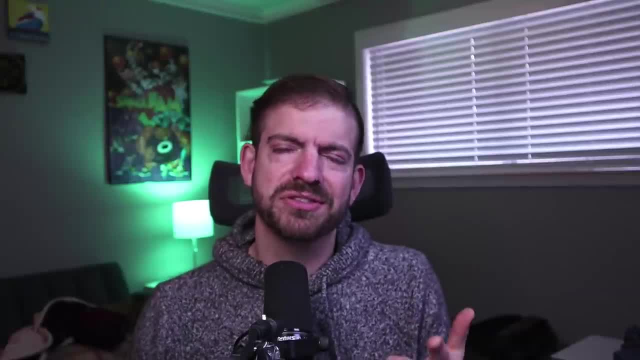 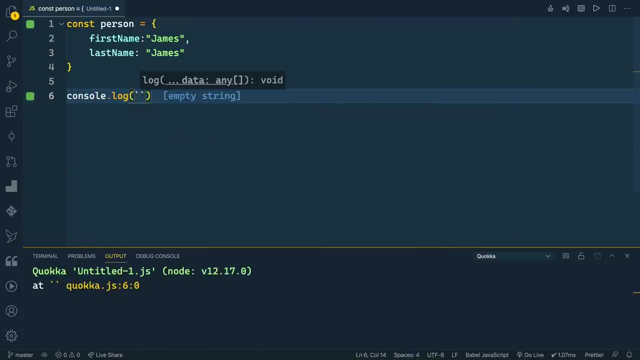 So destructuring spread operator template literal strings. these are so handy I almost I almost never use regular double quotes or single quotes are almost always always use backticks that allow us to do variable interpolation or string interpolation with our data inside of that ES6 template literal string. So those are ones that I use all the time Highly. 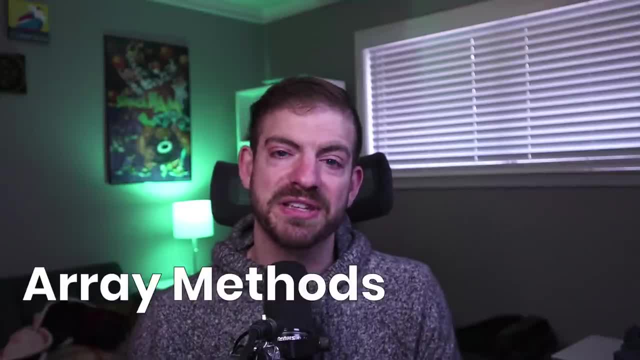 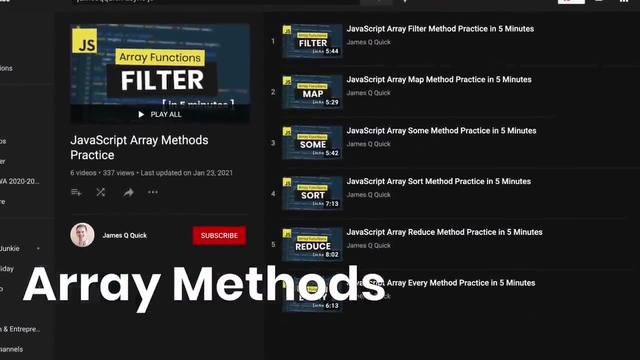 recommend you checking those out, All right. last up on this list is the array methods, And I started a series on these because of how important they are: Map, filter, reduce, sum, every sort. Those functions are incredibly useful, And it's stuff that you're going to see all over the place. 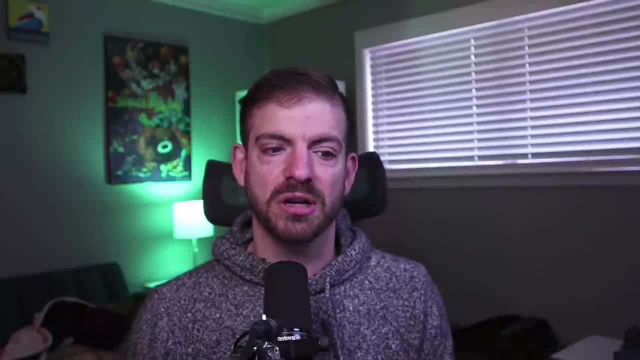 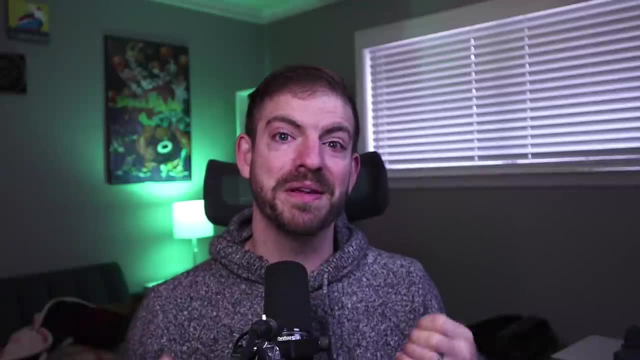 And, to be honest, some of the syntax with those are a little tricky, especially when you see them the first time, especially when combining them with arrow functions and the abbreviated arrow function syntax. If you've never seen an arrow function, if you don't know what an arrow function,